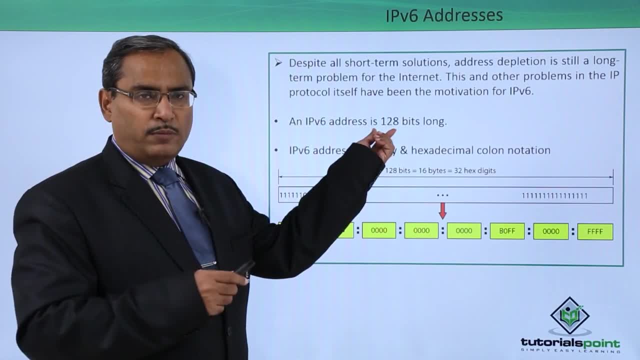 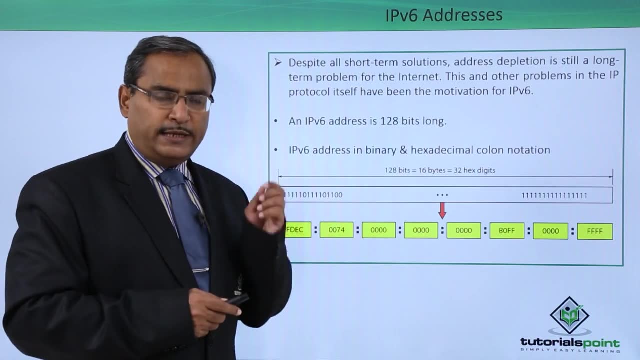 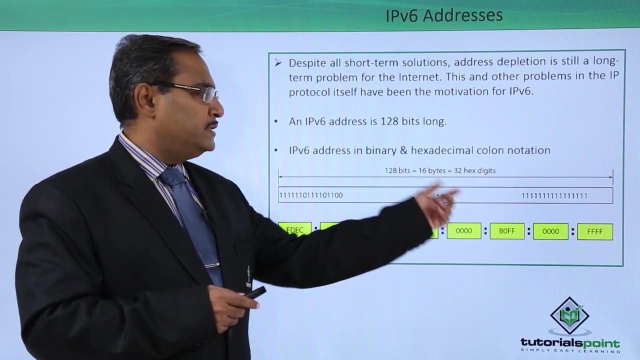 we are having 16 bytes, 16 into 8, if you go on multiplying you are getting this 128 bits. So IPv6 addresses in binary and hexadecimal will be represented in the colon notation. So just see here 128 bits. just consider you are having 128 bits here. It will be divided. 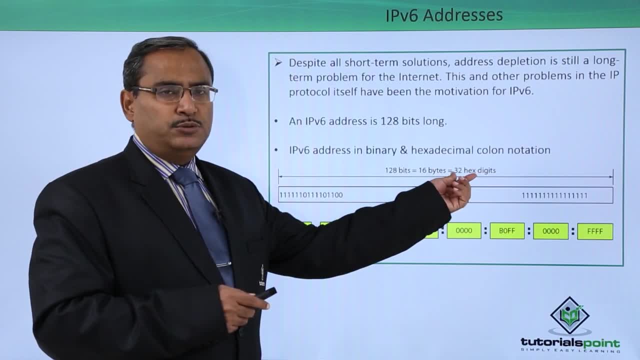 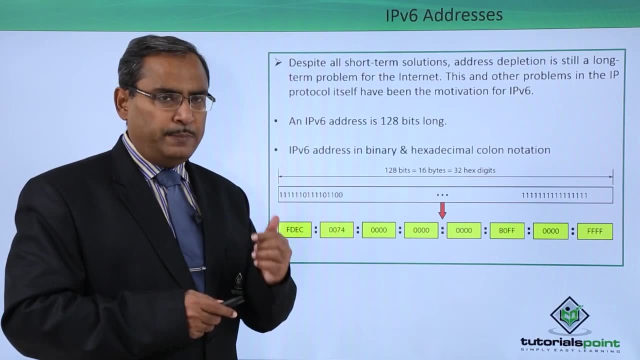 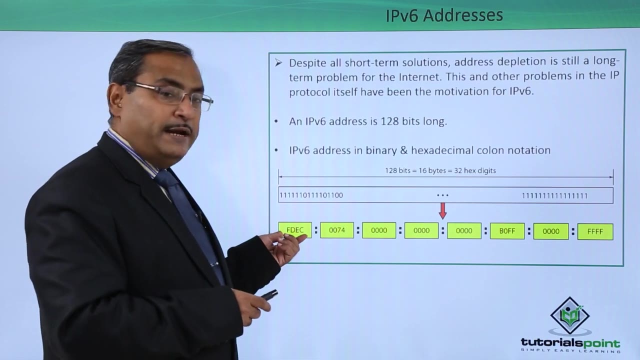 into 16 bytes. That means it will be having 32 hex digits, because 1 byte will have 2 hex digits, because hex digits are getting represented in the form of 4 bits or nibble. So that is why it is 32 hex digits and they will be expressed in this respective format, So 8 bits. 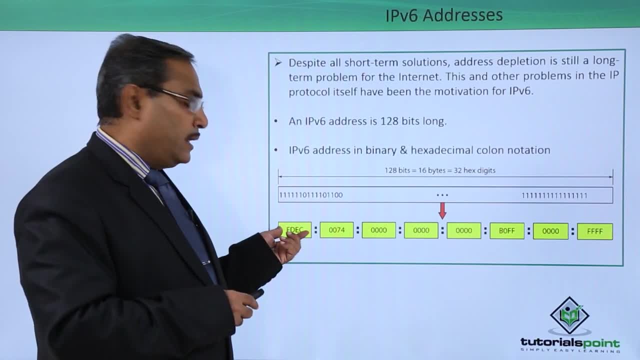 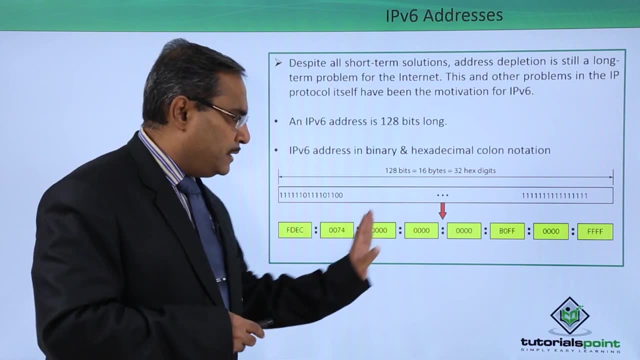 are there, So we are having here. we are having not 8 bits, we are having 16 bits there, So 16 bits, 16 bits. in this way, we are having 8 compartments and they have been separated by 7 colons. 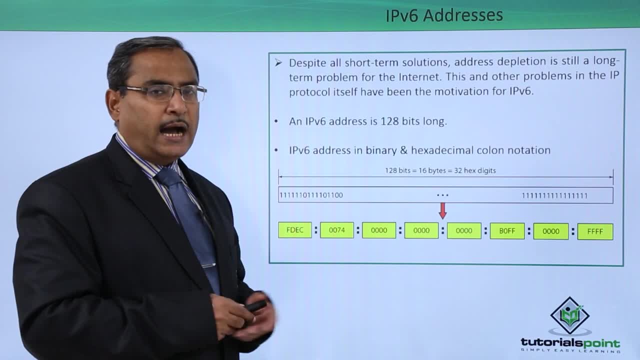 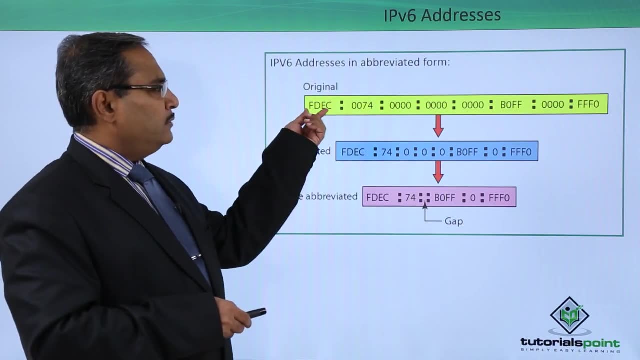 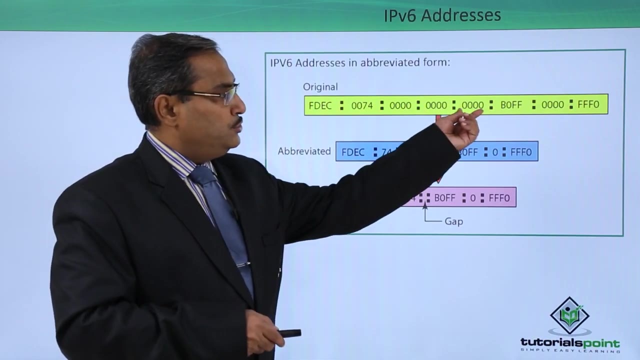 In this way we are having this representation. that is IPv6 format. So original address let it be this one: CEC, colon 0074, colon 0000, 0000, 0000.. You see, we are having all 0s there and then we are having some non-0 values. 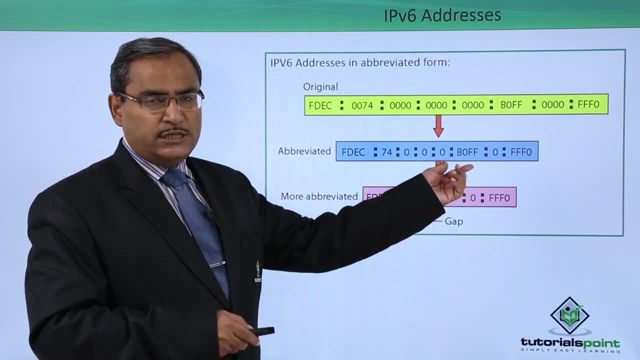 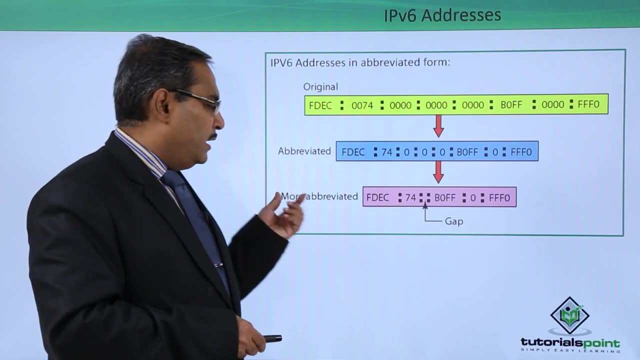 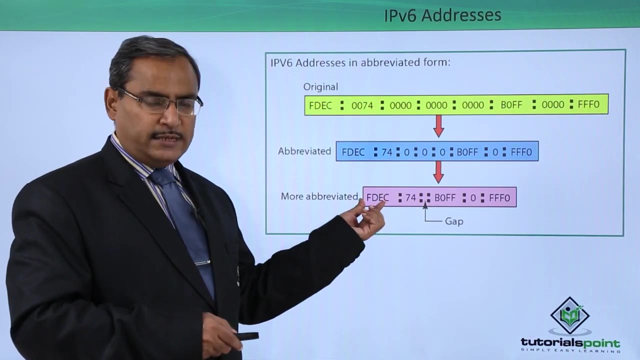 So what we can do, We can express it in this way, as usual. Otherwise we can put a gap. Otherwise we can put a gap. That means this is the respective, more abbreviated format. we are having this one. So now there is no confusion. We know that in this way, we are having 8 such sections. 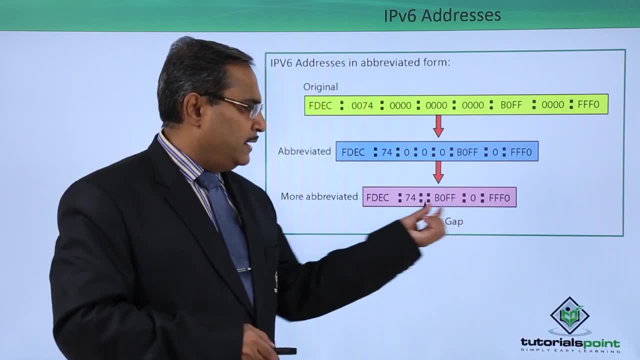 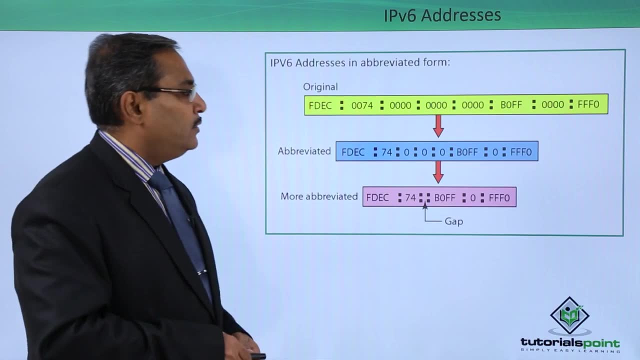 Fragments. So we are having 1,, 2,, 3,, 4, 5.. That means here we will be having 3 fragments will be there with 0 values, So that we can. if you want to go for the expansion also you can go for that, because 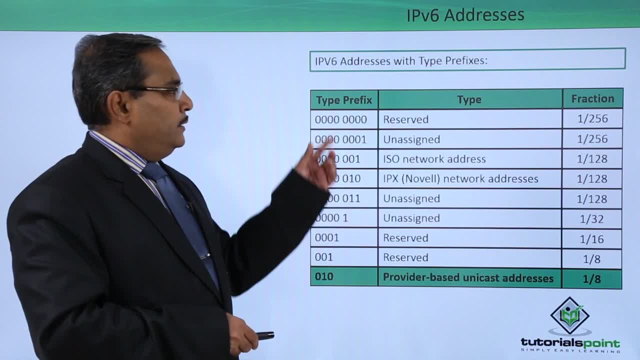 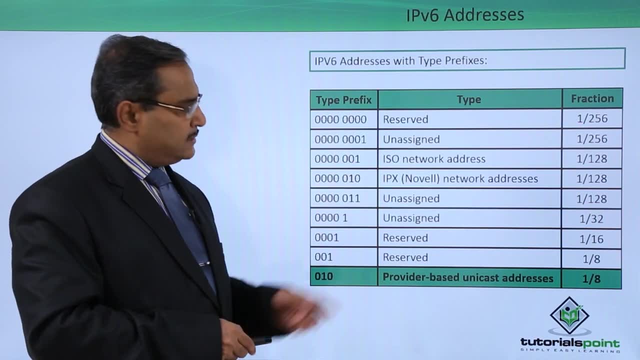 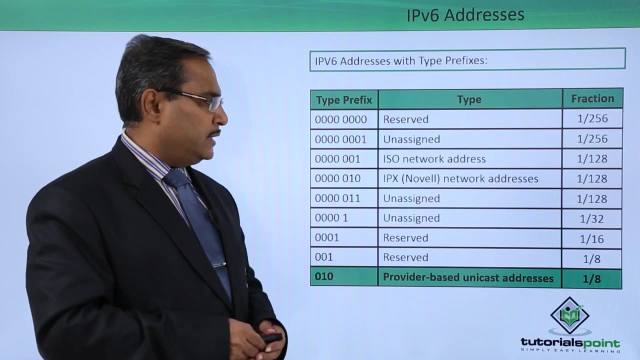 there is no ambiguity here. Now, these are the type prefix. These are the type prefix. So IPv6 addresses with type prefixes. So these are the respective type and these are fraction. So you can remember them, At least some of you. some of these combinations are to be remembered by you. You can pause the. 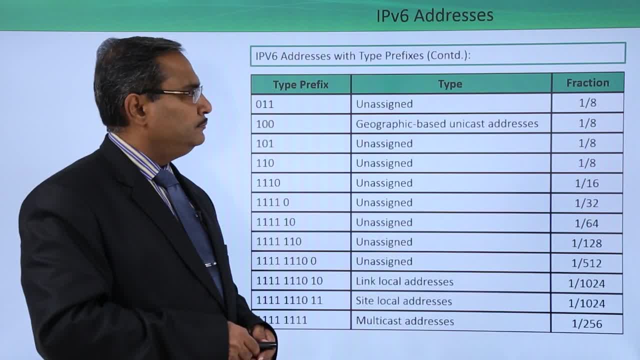 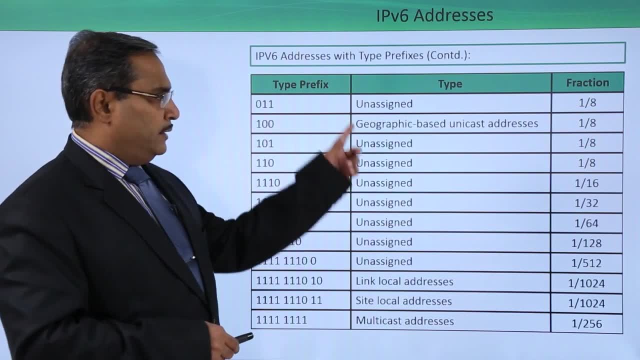 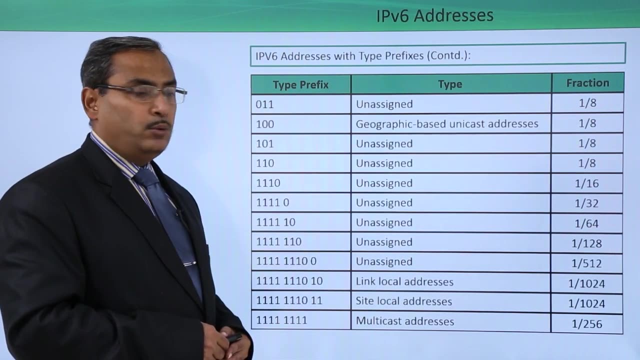 video. You can write it, Write them. So IPv6 addresses with type prefix. So here we are having the respective prefixes. are there Types, are there Fractions have been mentioned. If you can remember some of them, then obviously that will be good enough. Now we are having one example. 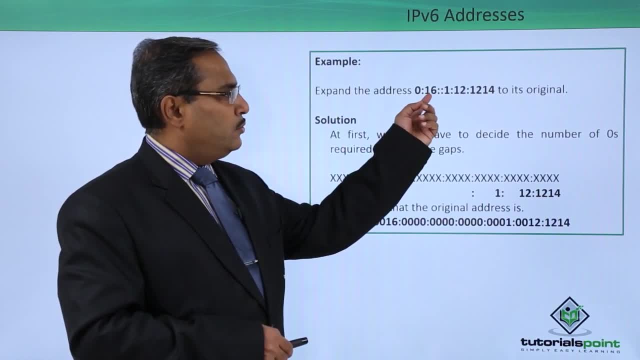 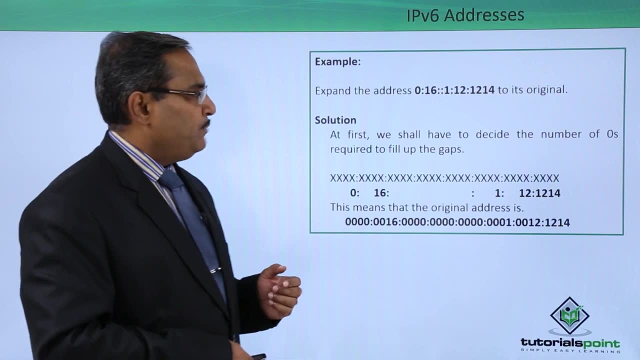 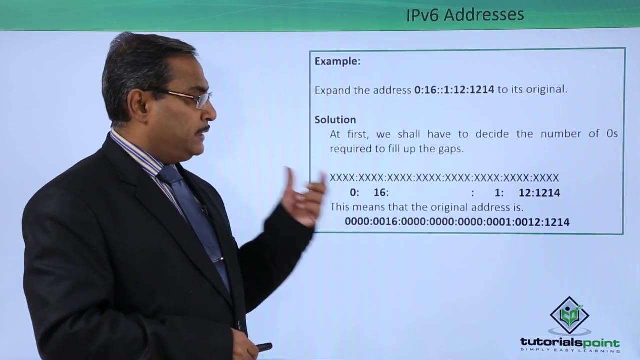 Expand the address 0, colon, 16, colon colon. So that is one gap here. So 1, 12 and 1, 2,, 1, 4.. Here we are having this, So we are having 1,, 2,, 3, 4, 5 numbers are there, So we are expecting that there will be. 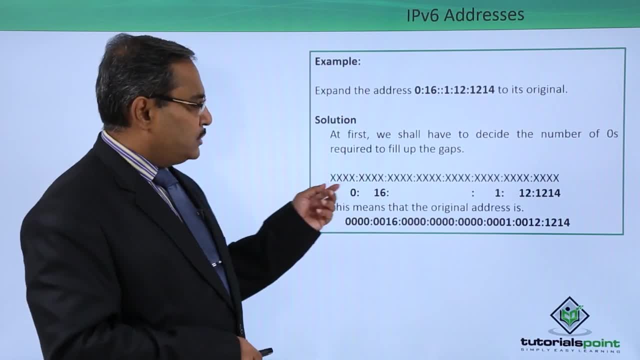 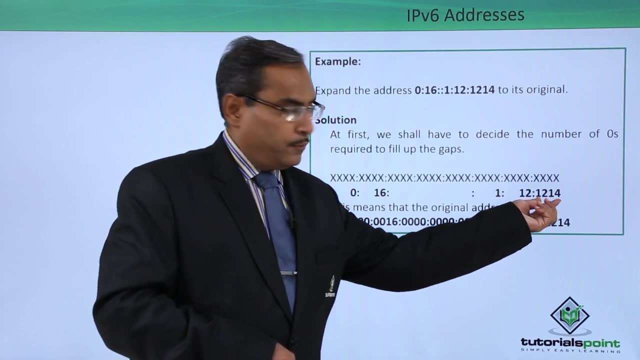 3 blocks will be there with 0 values. So that is why 0, colon 16, colon 1, colon 12, colon 1, 2, 1, 4.. So this is 1,, 2, 3. So there are 3 zones are there which will be filled up with the 0s. So in 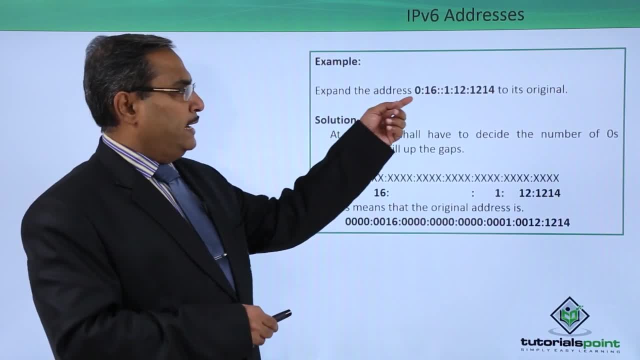 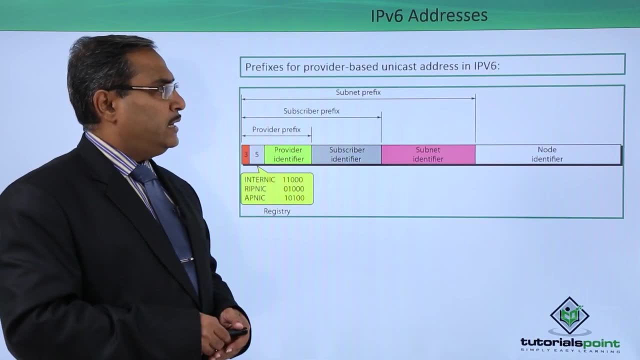 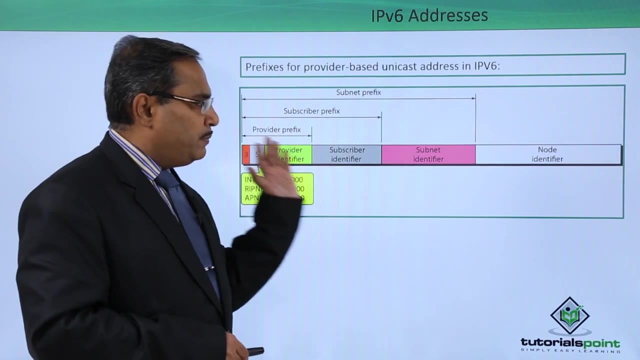 this way the original address can also be obtained if my address is in the abbreviated form. Now prefixes for provider-based unicast address, that is IPv6.. So this is the provider prefix, This is the subscriber prefix And this is the subnet prefix And last one is the node identifier. 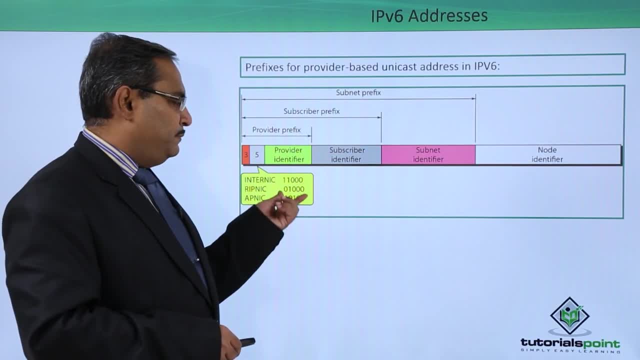 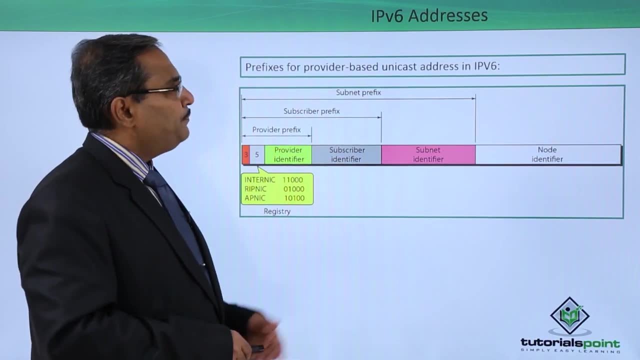 Here we are having 5 bits, We are having this 5,. 3 different combinations of this 5 bits for different sub-provider prefixes are there. So these are the respective registries. So this is IPv6 multicast addresses. These are the 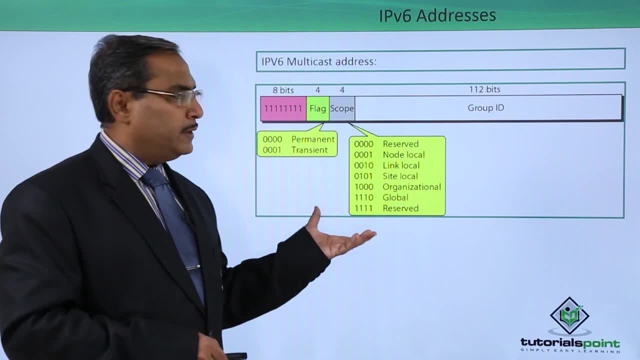 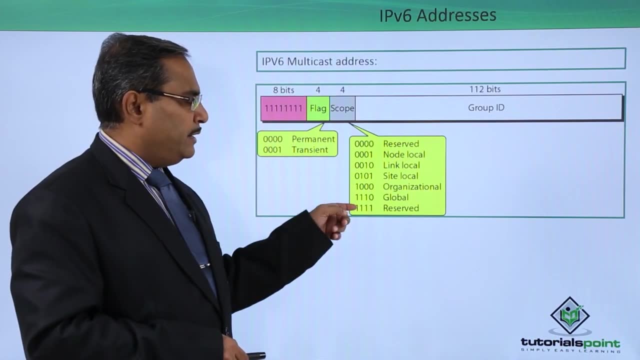 informative things are there. You are supposed to remember them because here we are having 4 bits. So these are the. these are the some combinations we are having. How many combinations? we are having 7 combinations of these 4 bits for different meaning And here for these flags. 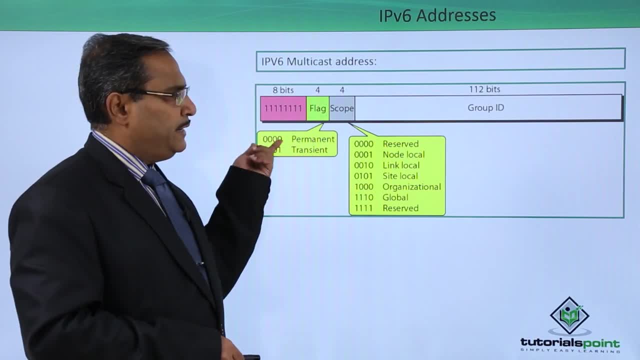 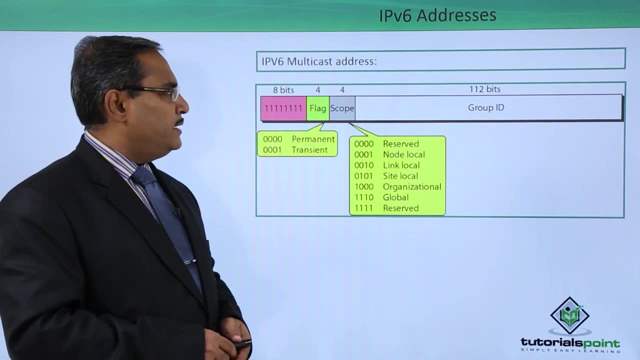 we are having 4 bits for the permanent And transient for this combination, bit combinations And rest 1 and 2 bits for the group ID. If you go on adding you are getting back your 128 number of bits. that will be there. 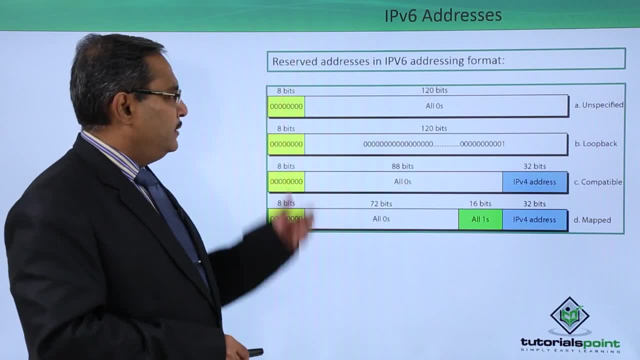 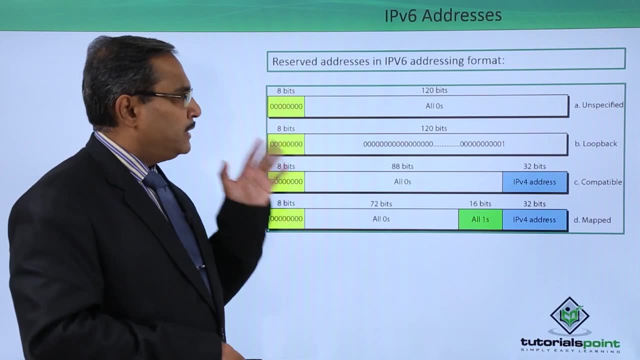 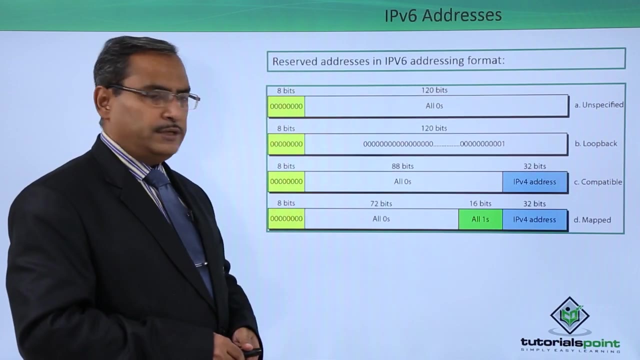 So reserve address in IPv6 addressing format. So it is for unspecified loopback, compatible and mapped. So these are the respective IPv6 addressing format, If you can recall, if you can remember. obviously you can produce it in your exam copy.